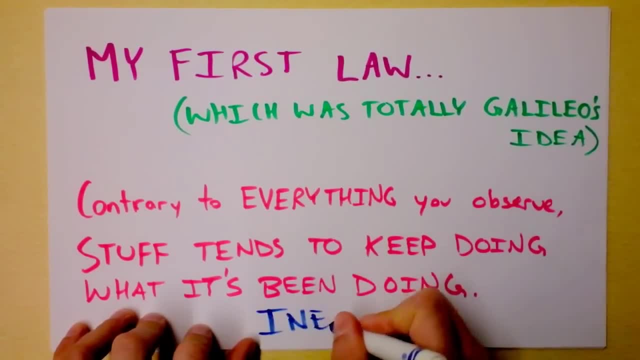 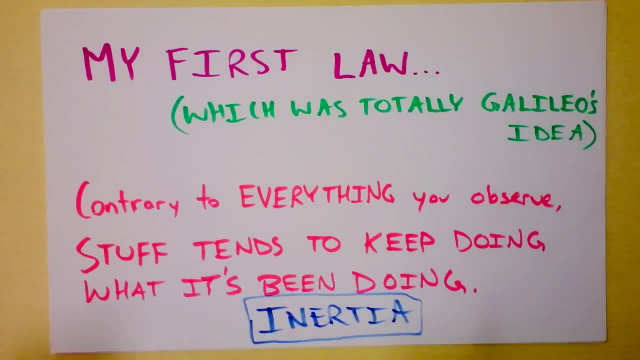 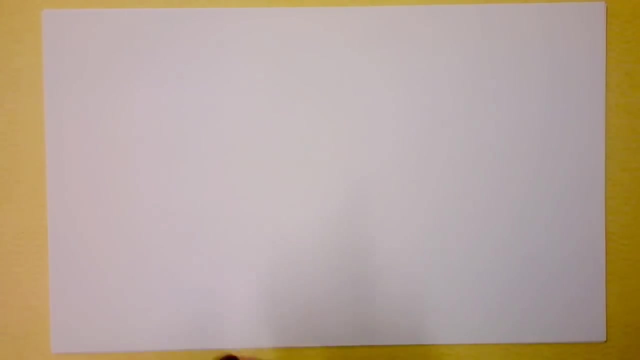 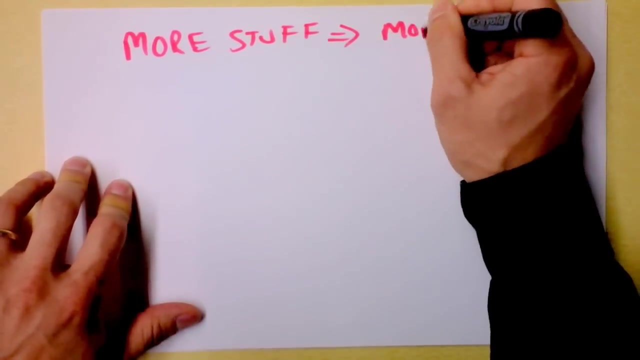 doing, And this concept is called inertia. This is the fat cat law. Inertia is the idea that stuff wants to keep doing what it has been doing, And inertia is connected to mass also. So what I'm trying to say is more stuff implies more wanting to keep doing, Wanting 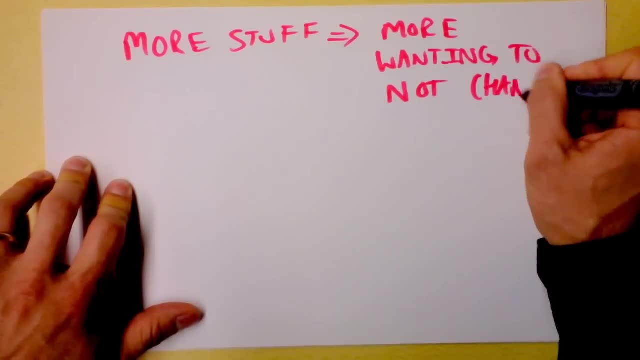 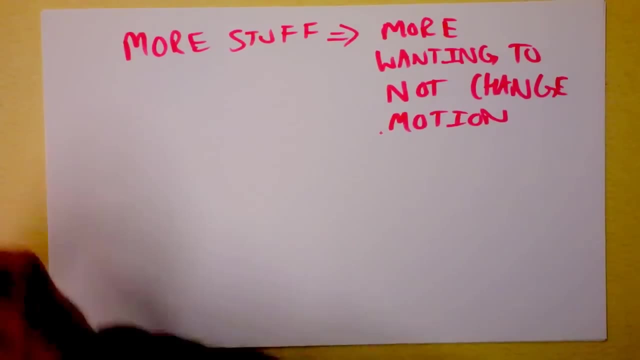 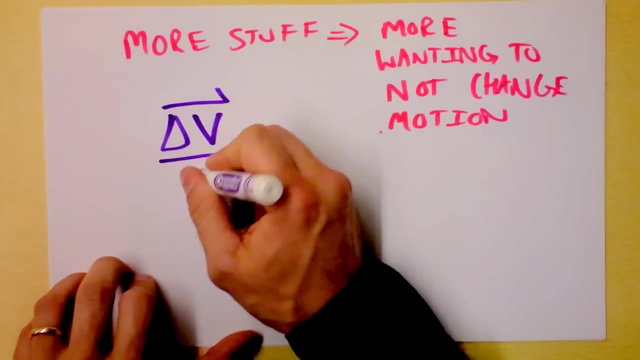 to not change motion. What the heck does that mean If something doesn't want to change its motion? can we get a definition of changing motion? Check it out. I'm thinking that might be delta V, the change in something's motion. But if I take delta V and divide it by delta, 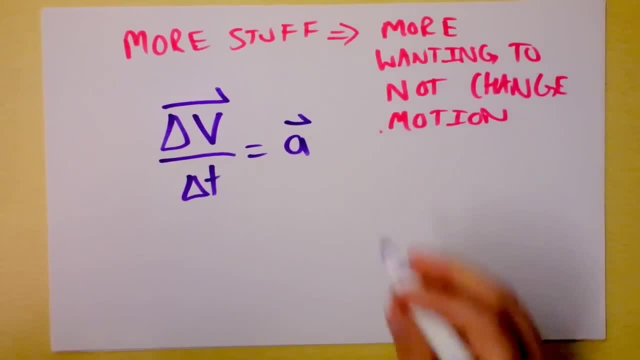 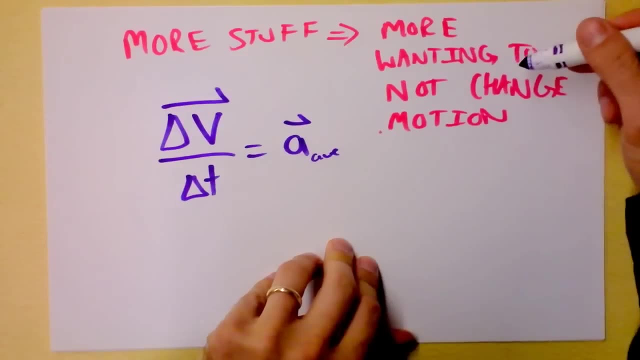 T, that sucker is acceleration. So that's kind of interesting. This is um. acceleration is change in motion. So I guess when I say more stuff, more wanting, more wanting, more wanting to not change motion, then I guess that's the same thing as saying more wanting. 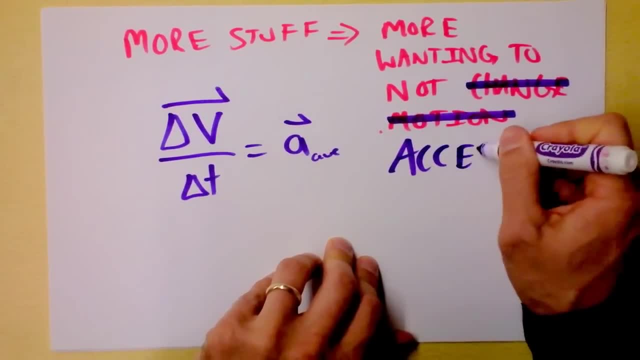 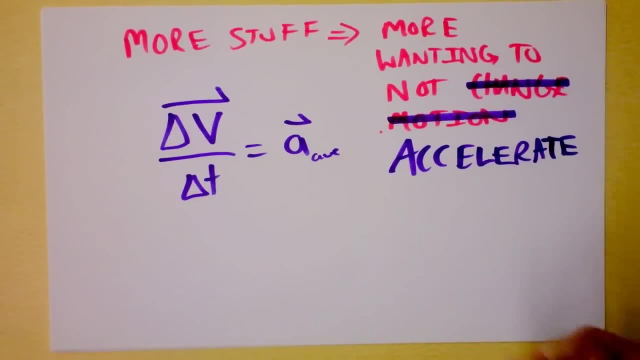 to not accelerate, And this will make a lot of sense when we get to my second law. But I want to point out how Galileo developed this. He said: listen, guys, you take this ramp and it's like that, And you put a, you put a marker on this side and you get it over. 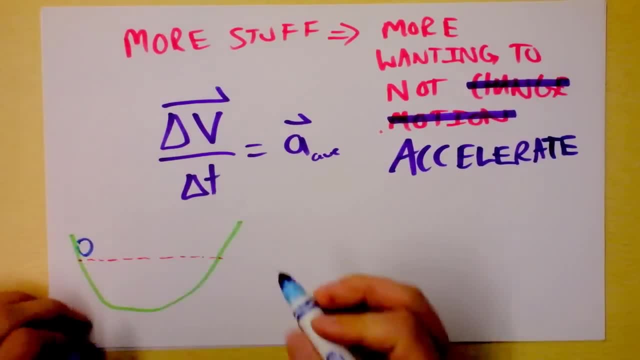 to the same side, same uh height over there, And you put a ball here, What's the ball going to do, yo? And and then everybody said, well, I guess if there's no friction it'll come back up to the same height. Of course that's kind of pretend. 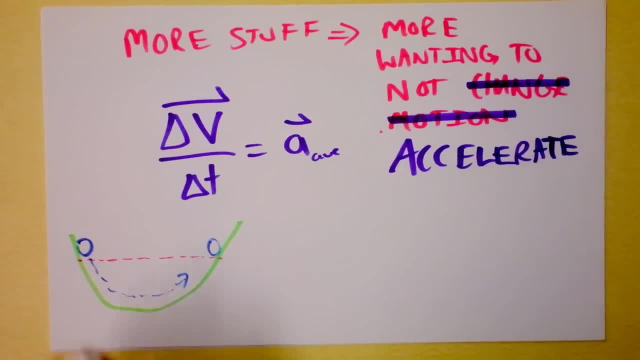 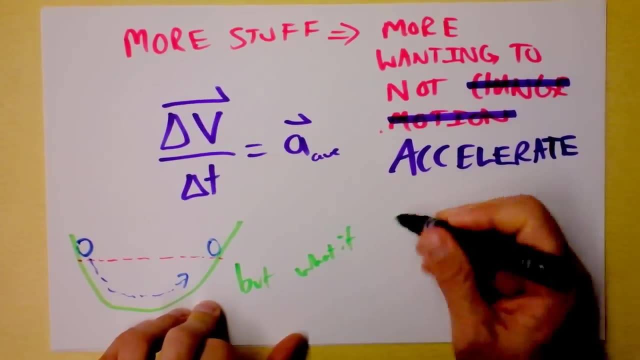 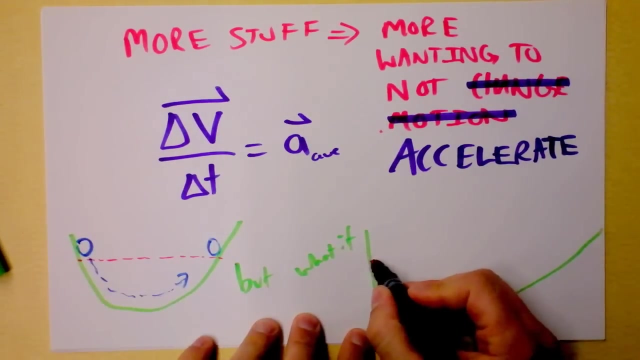 like maybe not a ball, Maybe it'd be easier to put a truck there or something. Um, and then, and then he said: but what if? what if it was like this? And then it was like that, afterwards would it still come up to the same height? And they reluctantly agreed: 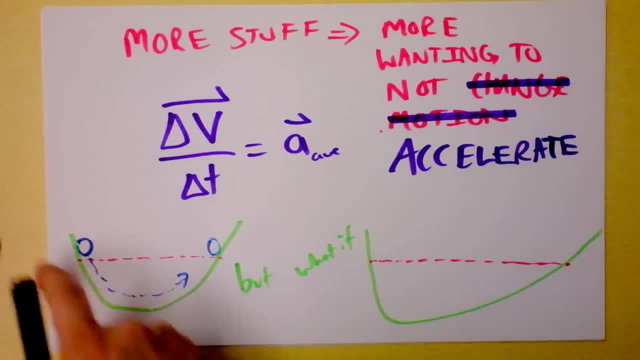 And perhaps you will also- reluctantly- agreed that if there's no friction at all, it's going to come back up to the same height. If there's no friction at all, then the ball will start here and go up to here, but it will take a longer time. So that's interesting, Will it? 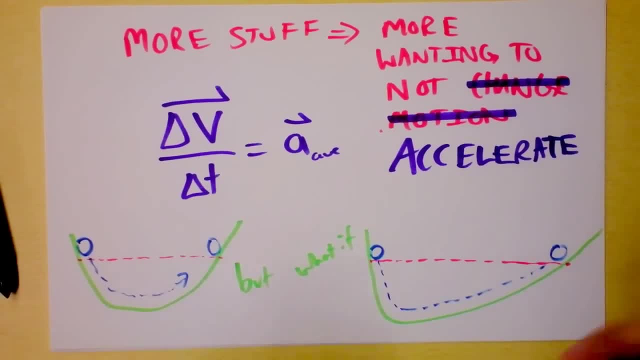 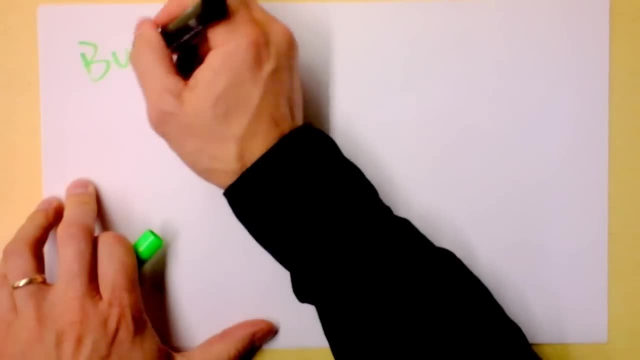 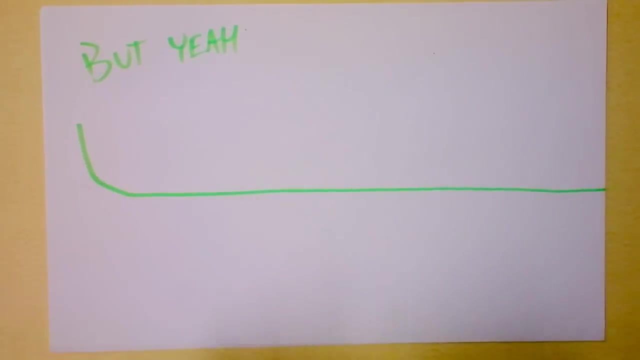 take a longer time? Interesting, I guess it would. And then, uh, what if so? Galileo goes on and says, but but yeah, what if the ramp goes like this? Whoops, I forgot to raise it up at that side.